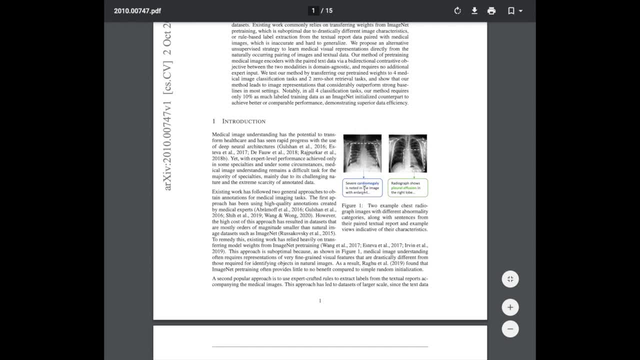 these chest radiographs and you have these short textual descriptions. so you use this contrastive pre-training task to align the representations such that this encoding is more similar with this text description than this image is. So once they pre-train with that, now they can. 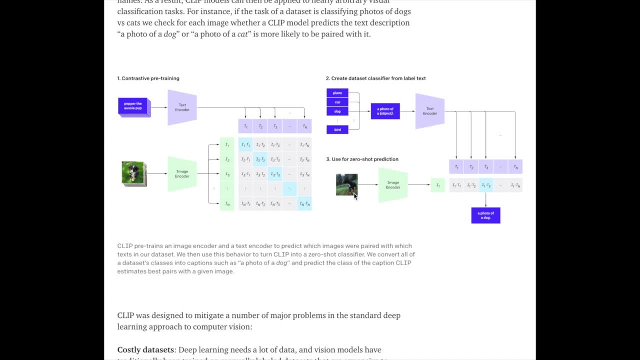 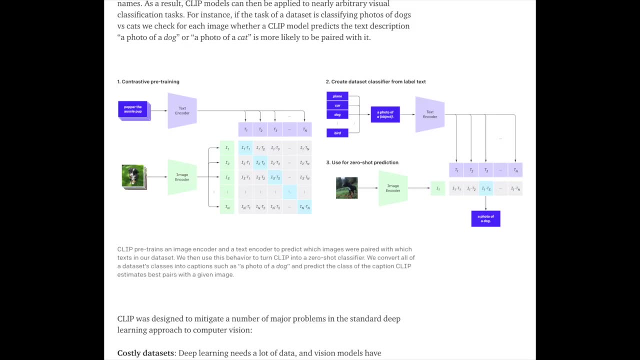 fine-tune. well, they don't even need to actually fine-tune with gradients, but they can transfer it to a new task zero shot, by using the same idea as pattern expression. So what they do is they insert a photo of a and then you just insert the object classes and now 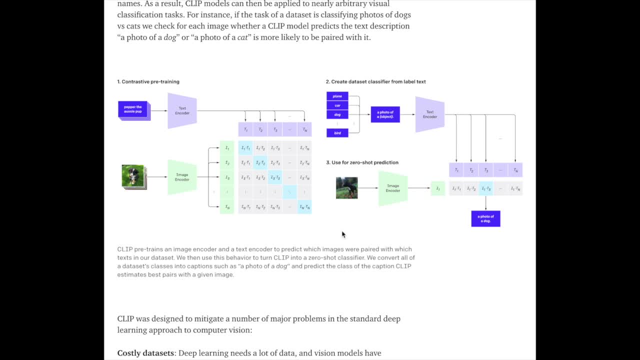 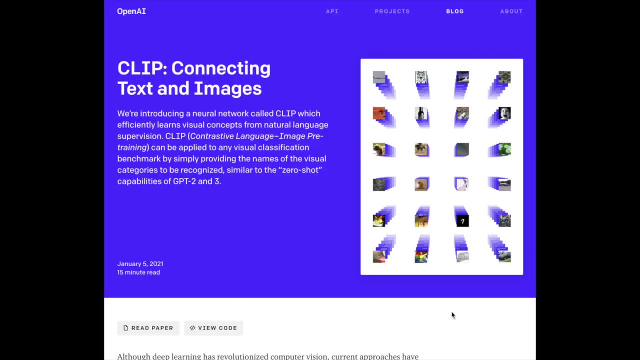 you turn it into the same kind of text similarity task as a contrastive pre-training task and allows you to do zero shot image classification. The blog post begins by describing some of the limitations of the current approach to computer vision and image classification models. Although models like 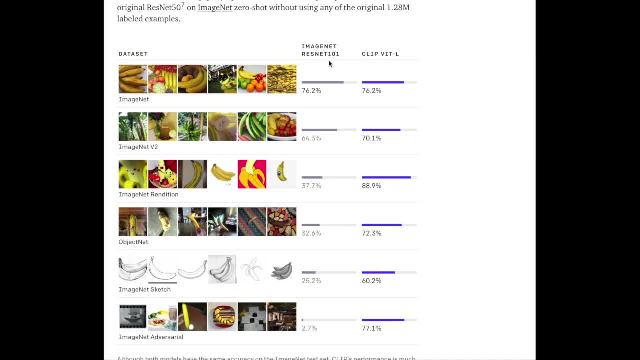 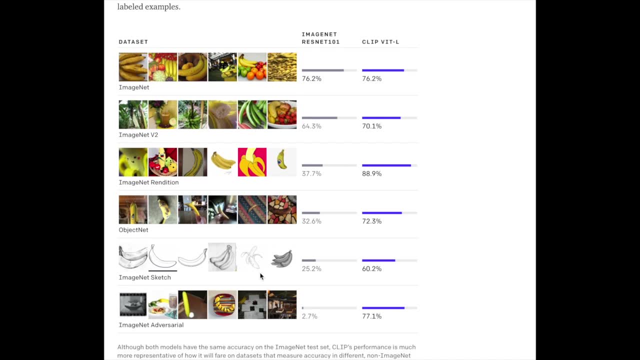 ResNet 101 or DenseNet or InceptionNet are really good at just the top five or top one percent classification accuracy. they fail to meet the requirements of the current approach. They fail with these modifications like the ImageNet A, ImageNet C, these robustness tests or adversarial. 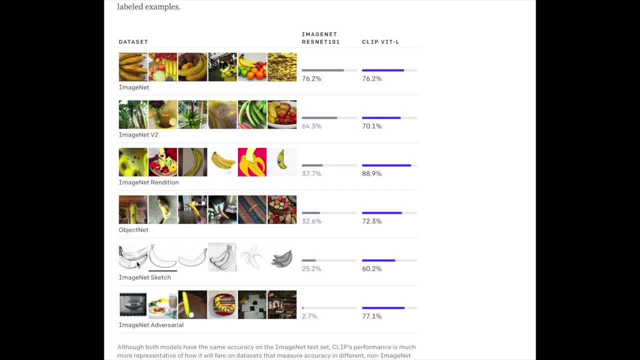 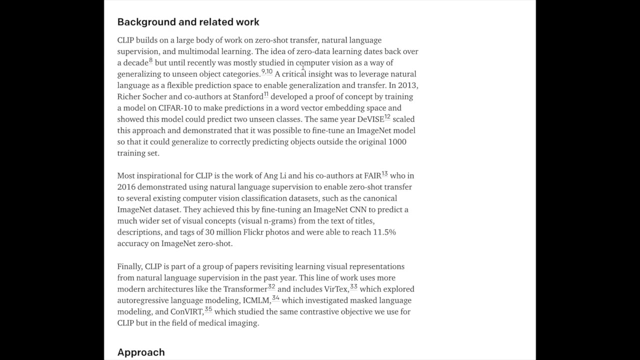 examples, as well as these slight differences, like ImageNet sketches that differ from the original ImageNet distribution compared to this clip contrastive task, which performs much better on these different kinds of data sets. The blog post continues to describe inspiration in vision, language models and the idea of a zero shot image classifier. They cite a lot of inspiration from 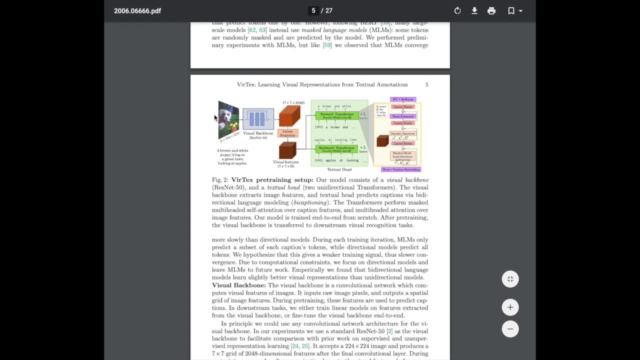 this work titled Vertex. In this case you use the visual representation, you encode this 224 by 224 by rgb image into a set of feature vectors and then use this to predict the caption. So this is one way of aligning the vision language domains to. 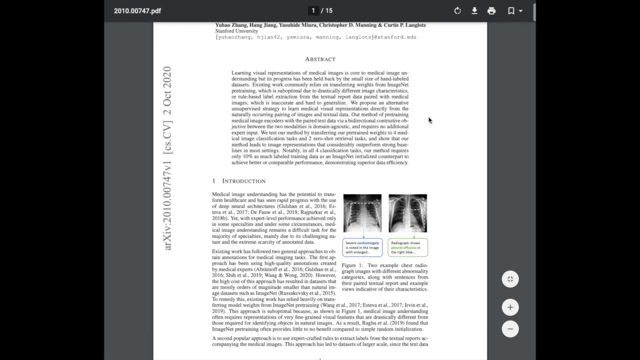 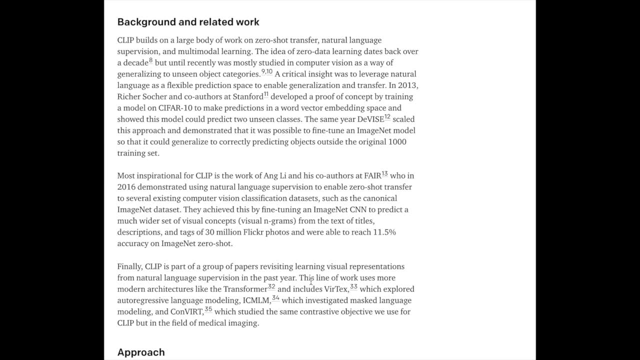 learning some kind of vision language representation, and then this convert paper is another way of doing it, with a contrastive learning objective. So they cite some of the previous works that have inspired this work, like Vertex and Convert, to try to align the vision and language representations. 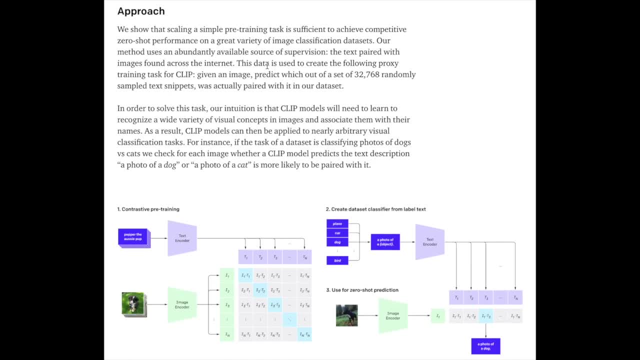 So we begin with this video by quickly walking through how this works. But some quick details on the approach. They are particularly using a batch of 32,768 of these text snippets to be paired with 32,768 images. Then you have the pattern exploiting. 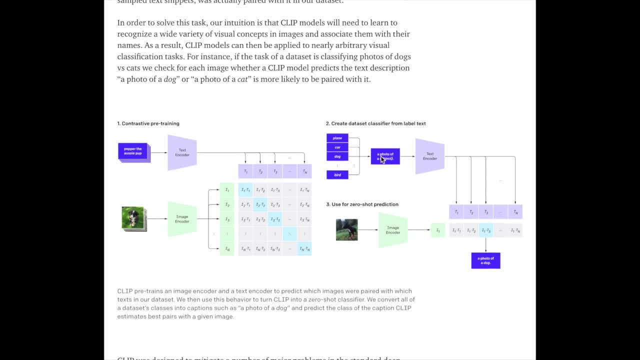 training, where you transfer this to the zero shot task by inserting a photo of a and then you insert the different classes. So this is the pattern, a photo of a blank. So they describe some of the other problems that CLIP is able to solve that are currently hindering, say, 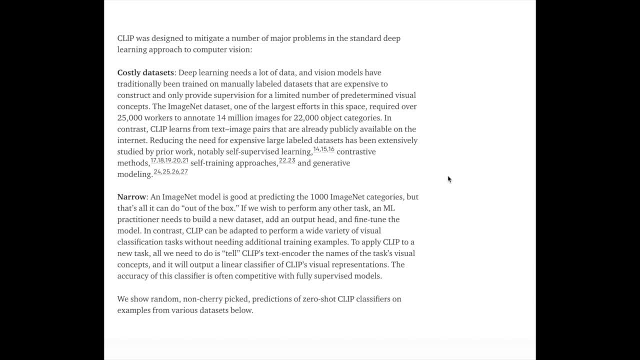 training a ResNet on ImageNet. The first problem with the previous approach to image classification is these data sets are really expensive to build. The ImageNet data set requires over 25,000 workers to annotate these 14 million images over 22,000 object categories, So employing 25,000 people to 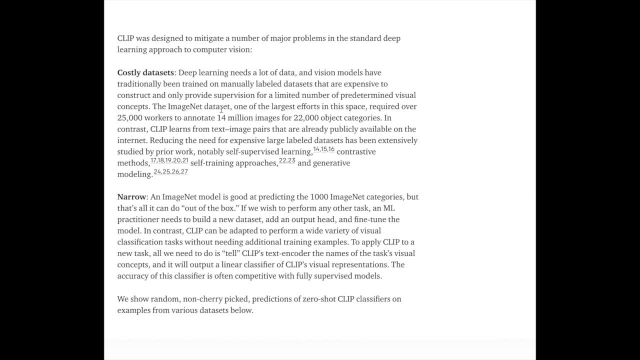 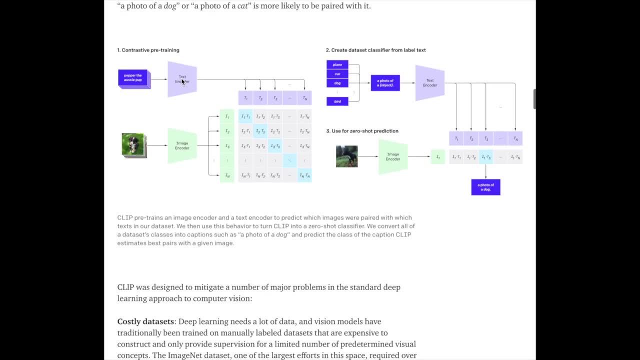 do. this is a really expensive way to construct these labeled data sets And lately we've seen a lot of self-supervised learning that's able to learn representations from unlabeled data, like contrastive learning tasks to learn a representation just by scraping the internet, rather than having 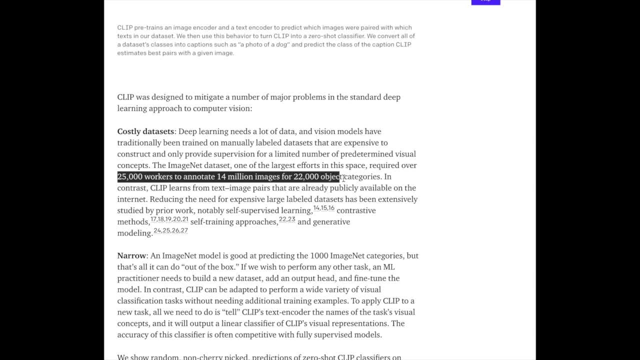 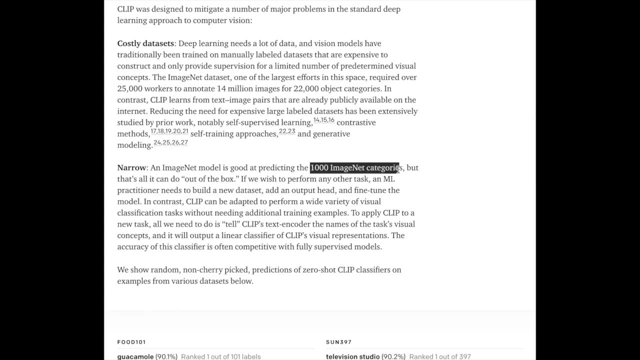 to say, deploy 25,000 workers to annotate 14 million images or this kind of expensive effort. And the next thing is that the ImageNet model is pretty narrow. It only knows these 1,000 ImageNet categories but it can't generalize in the same way that CLIP can just generalize by inserting a new. 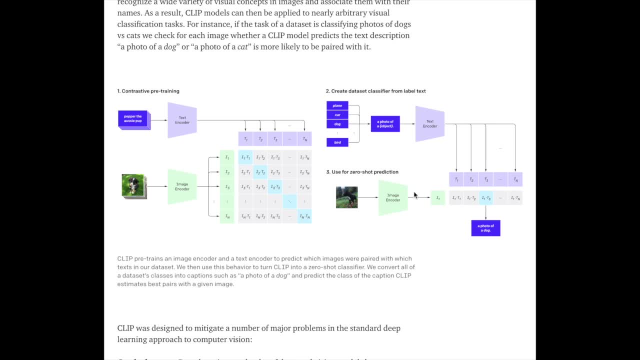 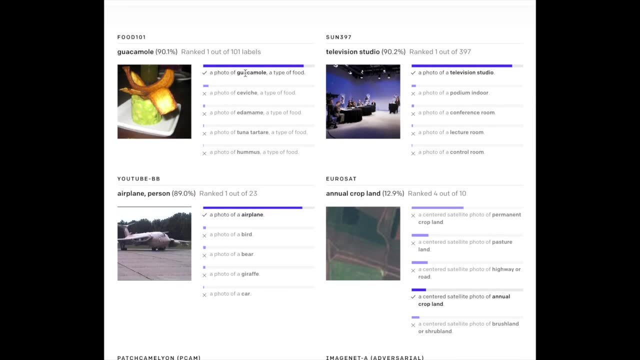 kind of pattern to transfer it to this new task. So then we see some more. they say random, non-cherry picked examples. So here's an example: a photo of guacamole, a photo of ceviche, a photo of edamame, and you see how this. 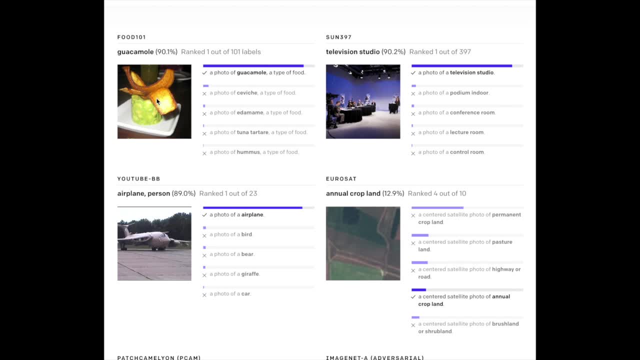 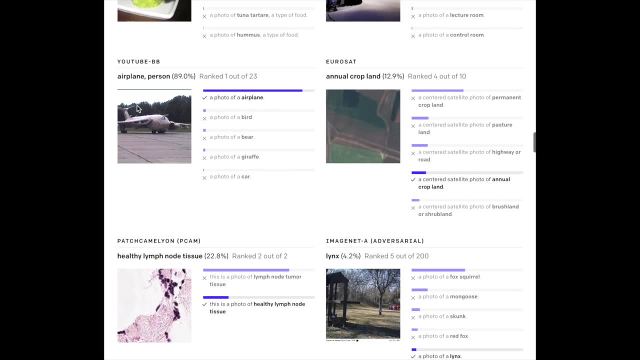 pattern explaining training is adapted to have this text similarity class or text image matching task with these images and then these text prompts And they see the same case here: television studio and these other examples and you can see show more if you want to see more of these examples. 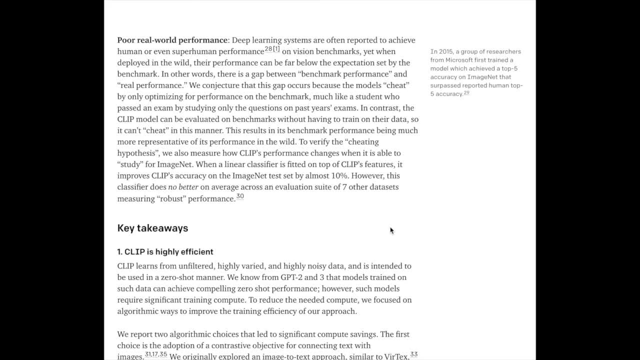 on the OpenAI blog post. They cite one more issue with having this supervised learning training set and say fitting a ResNet on this supervised learning set. The problem is that this training set isn't really representative of the performance because it's essentially memorized or cheated by training on this data set, compared to these zero-shot models. 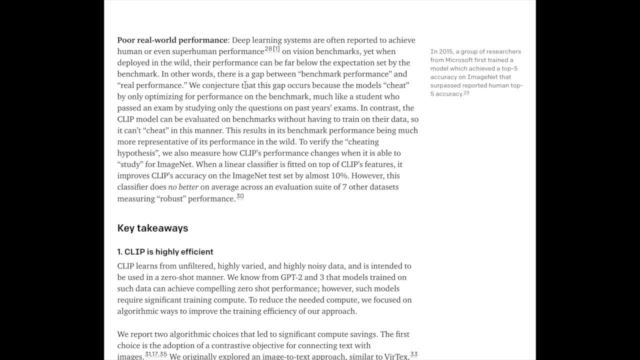 that they by design they can't have memorized the data set because they don't do any training on this data set. So they also show that when you do study for ImageNet or you know, fit the linear classifier that has gradients on top of the features that are extracted from the CLIP model. 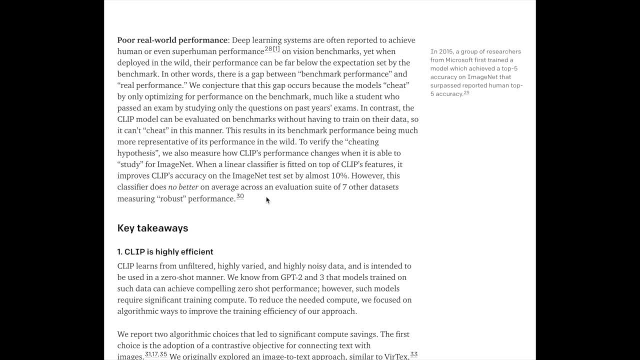 it does improve the accuracy by almost 10 percent. but and then, as they show that this robustness test is still not hindered- compared to these other kind of models of supervised learning that study or memorize the original data set. So some of the key takeaways are that the CLIP model is highly 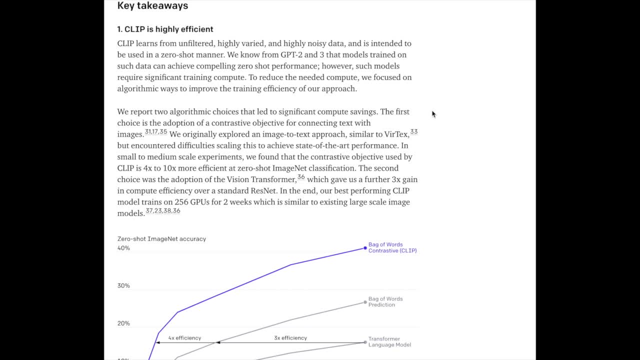 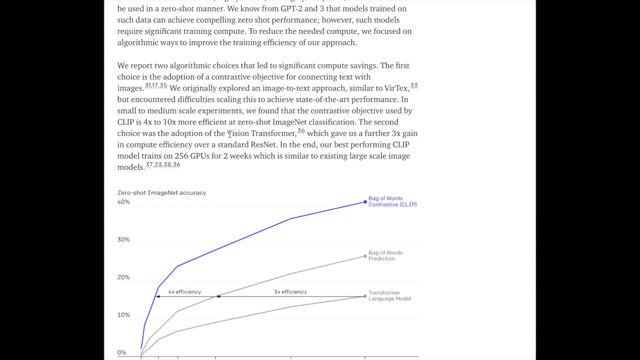 efficient, particularly in addition to using this contrastive learning objective, which is different from the image to text approach in the vertex model, where you encode the image and then predict the text caption from it. compare that with this contrastive similarity matching task. It's more efficient. in addition to that, they use the vision transformer, So the vision 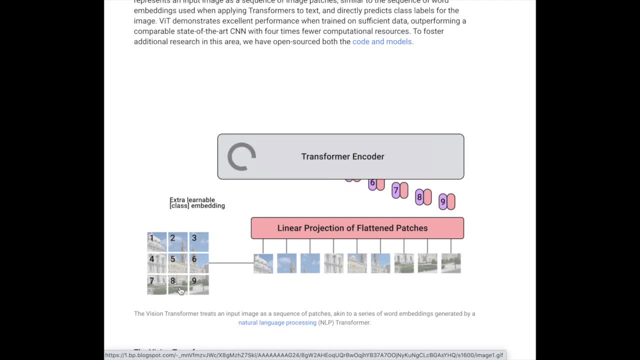 transformer is this model developed by Google, compared to ResNet, where you just take this whole image and then pass it through this sequence of convolutional blocks with skip connections. This vision transformer breaks the image up into multiple patches and then it treats that patch as as if it's like a sequence of tokens for natural language processing, and then it will use the 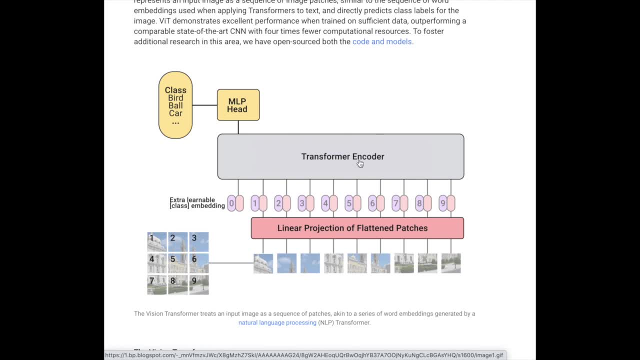 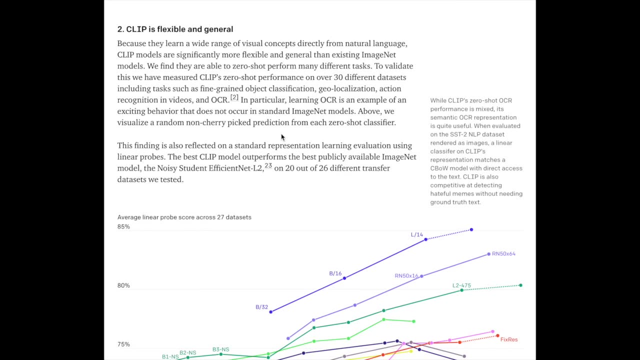 position embedding, like in the transformers, use the transformer encoder the self-attention layers stacked together to perform computer vision tasks. The next takeaway is that CLIP is flexible in general. so they talk about additionally testing CLIP on fine-grained object classification, geolocalization, action recognition and videos and optical character recognition, So particularly 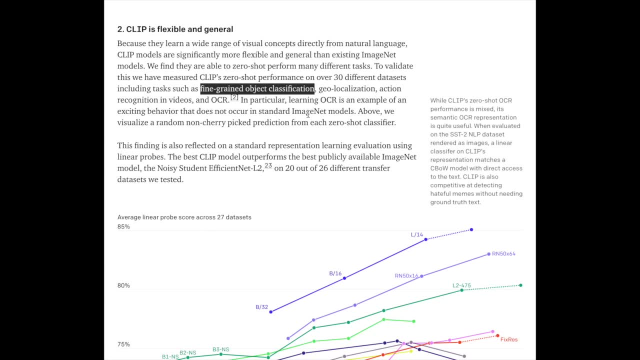 fine-grained object classification would be. there's some data sets- I think it's called like Stanford cars, where you're not just classifying broad categories like CIFAR 10, where CIFAR 10 is, say, like very different things, like cat, dog, truck, airplane, frog, compared to, say, a data set of cars. 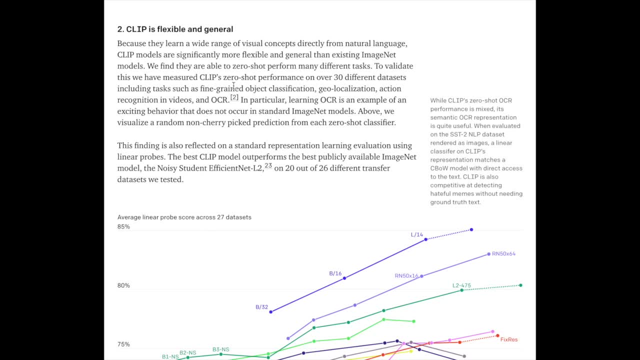 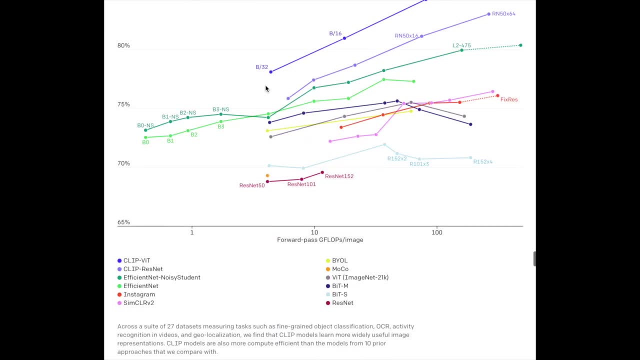 and then you're classifying the specific type of the car. So that's the difference between, you know, fine-grained object classification and they're showing that CLIP is able to do this flexibly with this pattern exploiting framework just pre-trained on the on the internet pairs of 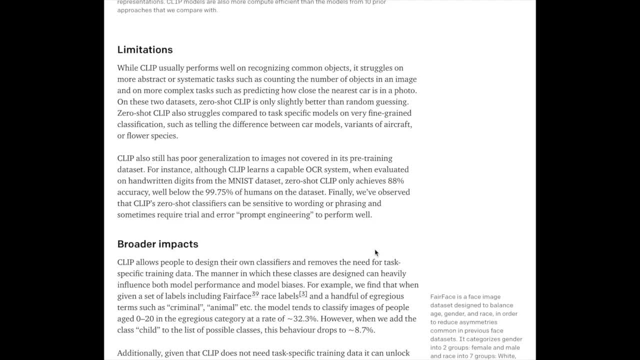 text and images. Finally, they do bring the CLIP model down to earth a bit, with some of the limitations. One of this is that it fails at these complex tasks like counting the number of objects in an image or predicting how close the nearest car is in a photo. So, on these more complex tasks, 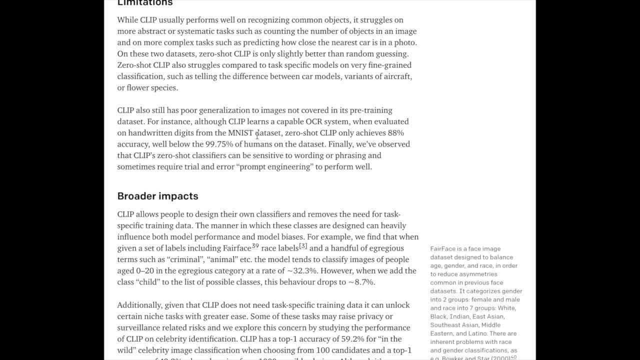 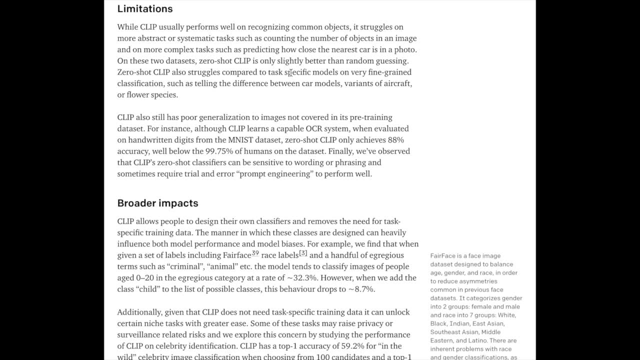 and then further they cite that it doesn't perform as well on, say, the MNIST data set, as training on the MNIST data set would do, even though that's back to that original discussion on kind of memorizing, studying or kind of overfitting to the test set with the train set. So 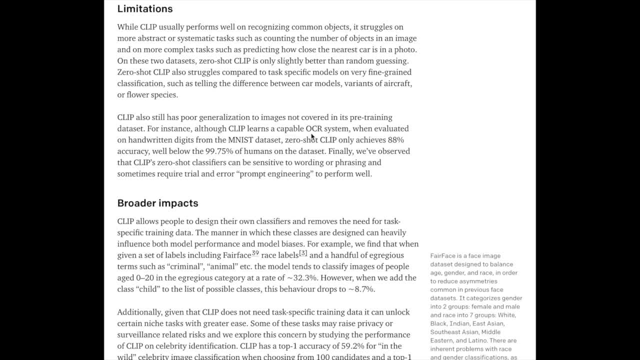 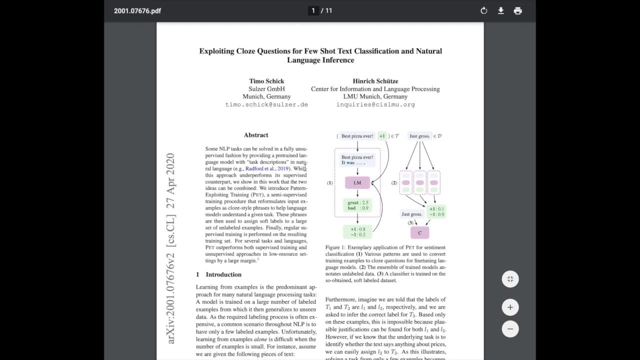 zero-shot CLIP still achieves 88 percent on MNIST. and again, to adapt this with something like the pattern explaining training, which is how you adapt CLIP, to some kind of downstream task, you'd say: take an image of the MNIST digits like one, two, three, four, five, then you'd say a photo of 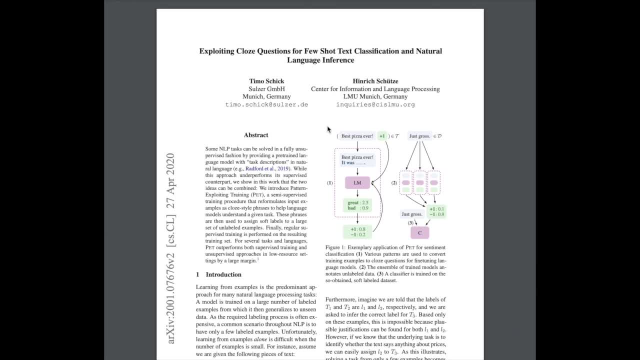 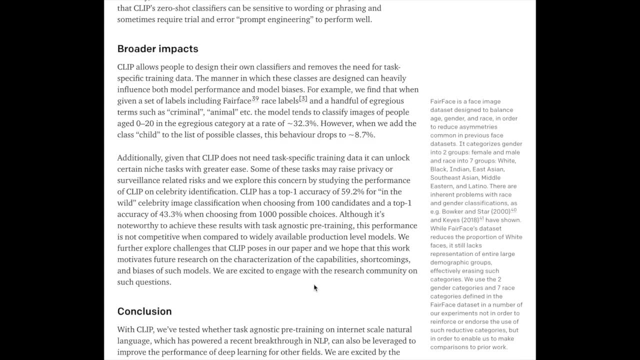 a, and then you have the text matching for a photo of a one, a photo of a two, a photo of a three, a photo of a three, and then it would have some kind of matching score for each of those text patterns. The authors report some of the broader impacts, like the bias that can be present. 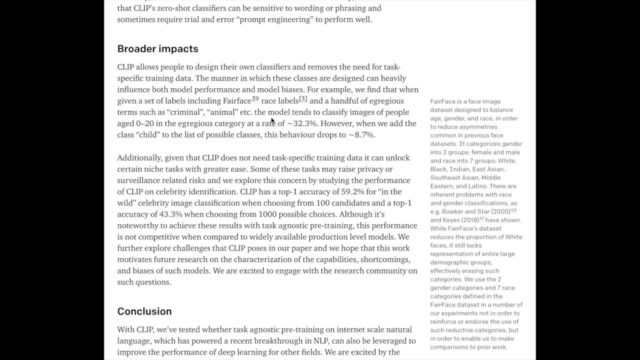 in the data when it's scraped from the internet to do this representation learning. They cite how, when you're pairing images of people age 0 to 20, they're more likely to be affiliated with language terms like criminal and animal, and then they show a potential solution to this by adding the class. 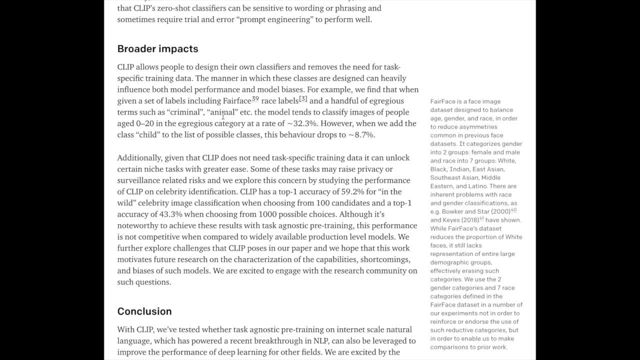 child to the list of possible classes alongside, say, criminal and animal, if these are the two, uh like classes to insert in some template of this is a photo of a mask and then the mask is where you insert the object class labels. Then further they describe a problem of celebrity identification. 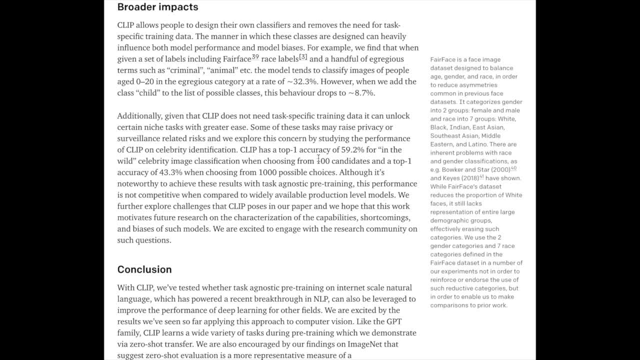 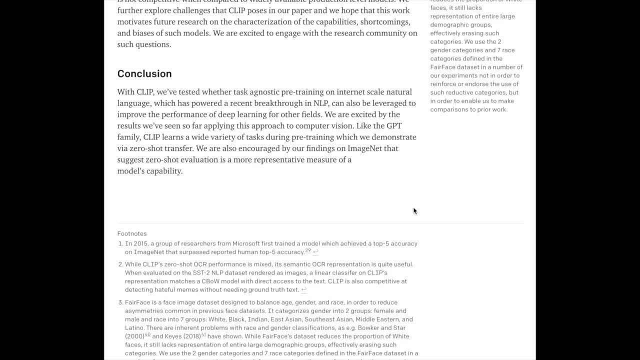 that this is able to do celebrity identification right off of the shelf and you don't need to have too much of a training set in order to do this task. So, all in all, this is the new CLIP model developed by researchers at OpenAI. This is a really exciting new approach to using contrastive